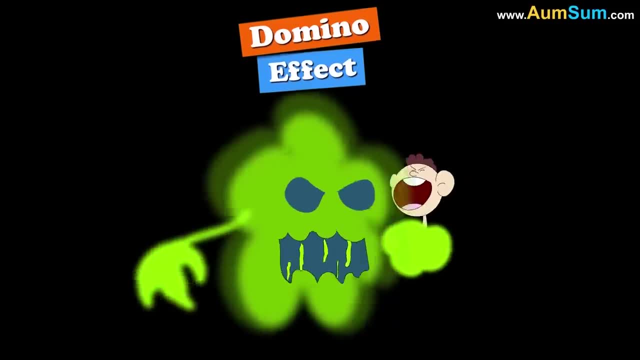 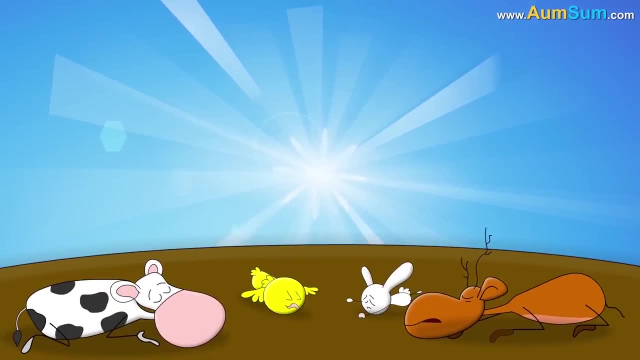 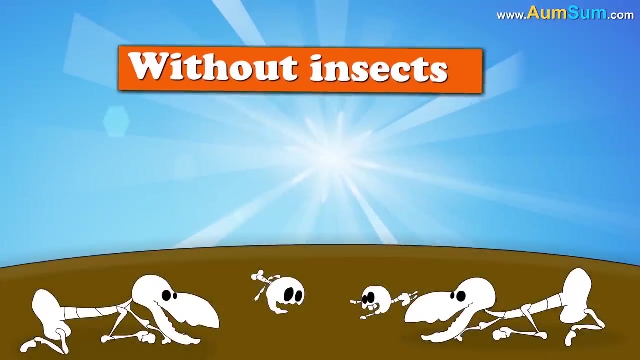 Finally wiping out the top of the food chain, that is, human beings. Also, don't be surprised if you suddenly see a lot of dead things everywhere. This is because insects are decomposers. Without insects, decomposition process would take much longer. 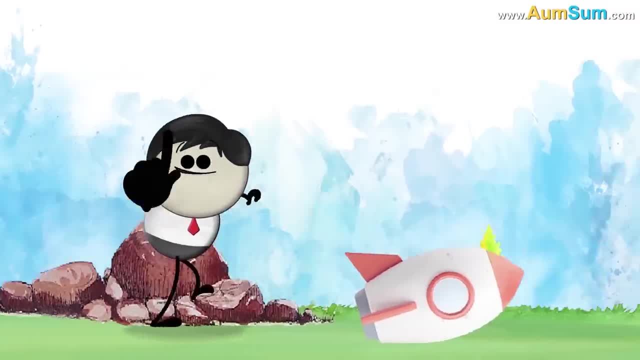 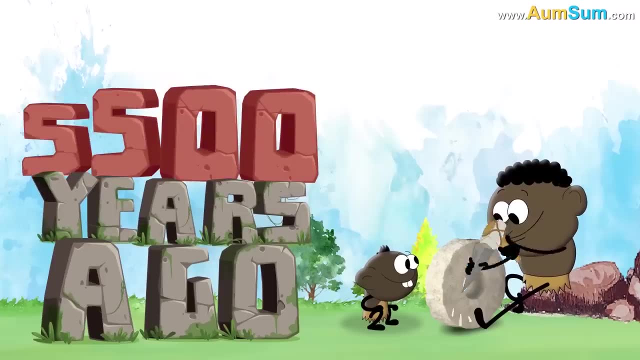 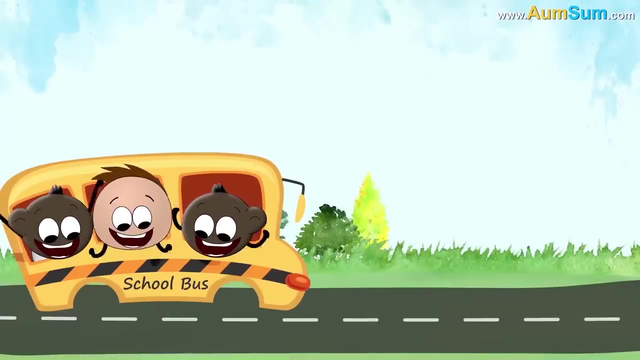 What if wheels were never invented? No problemo, I will just use my private rocket. Oh AumSum. Wheels are believed to have been invented almost 5,500 years ago. Ever imagined what the world would be like without wheels? How would you go to school, work or even on a holiday? 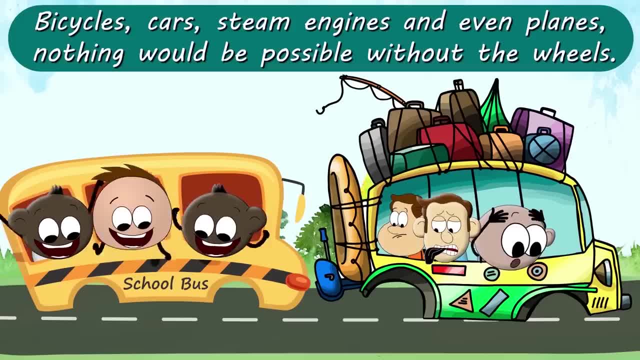 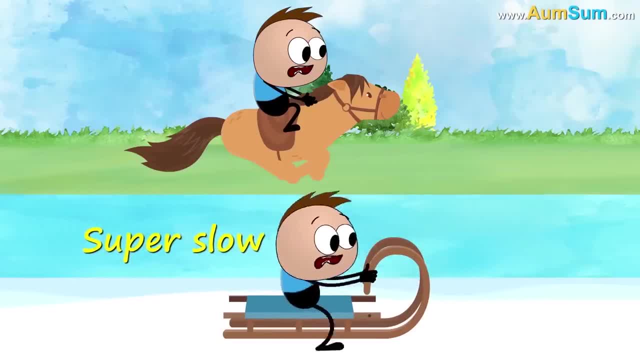 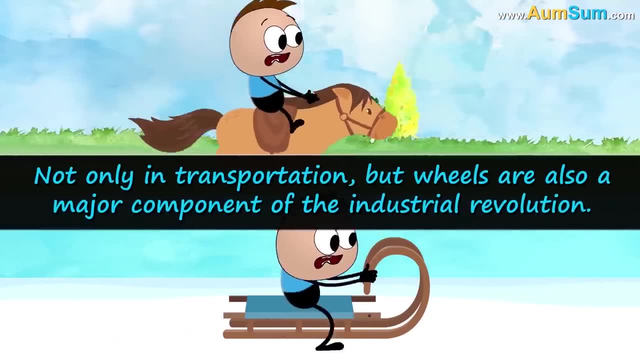 Bicycles, cars, steam engines and even planes. nothing would be possible without the wheels. Yes, horses and sledges would be there, But it would be a super slow and super rough ride. Not only in transportation, but wheels are also a major component of the industrial revolution. 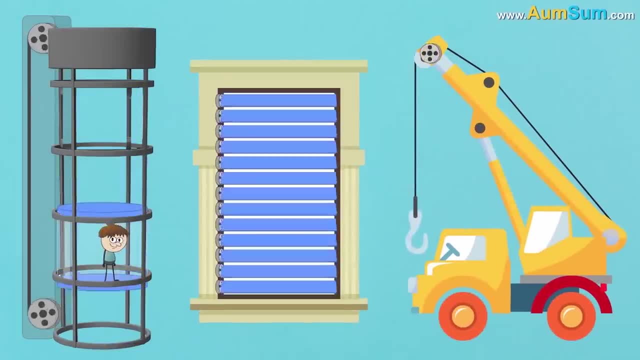 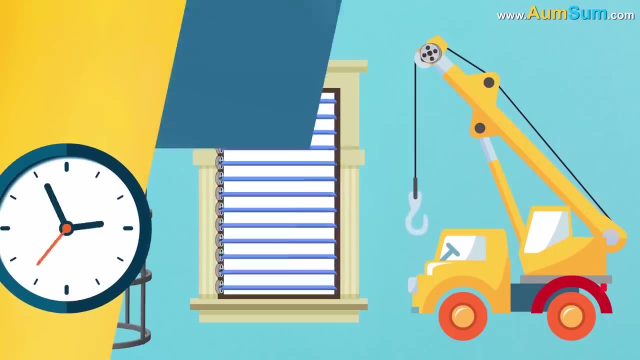 Elevators, blinds, cranes, etc. all have some form of wheel hidden in them. Now, on adding teeth to wheels, gears were invented. Clocks, grinders, car engines, bicycles and other complex machines worked with the help of gears. 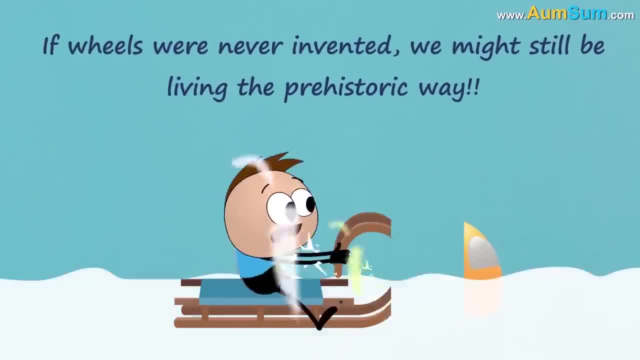 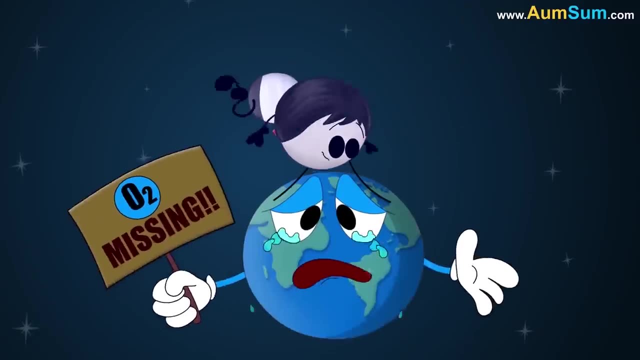 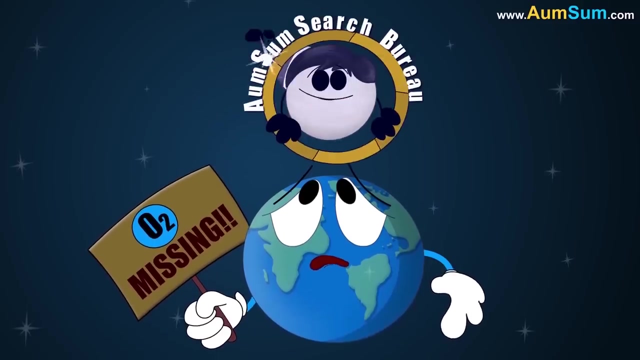 So basically, if wheels were never invented, we might still be living the prehistoric way. What if earth lost oxygen for 5 seconds? We would need to organize a search party. No, If it was just 5 seconds, we wouldn't notice changes in our breathing. 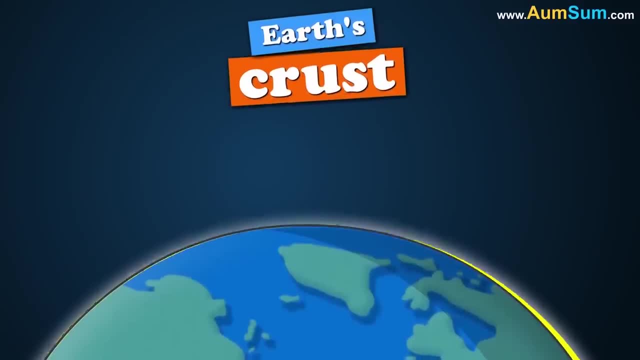 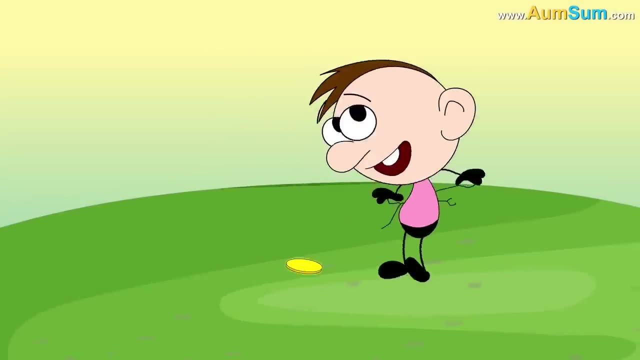 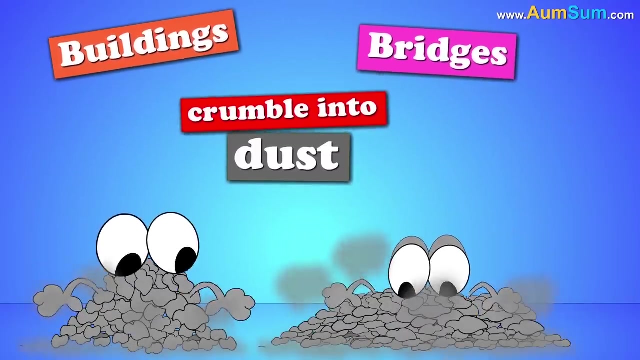 But do you know what would happen around us? Earth's crust contains 45% oxygen. Without oxygen, crust would crumble, causing the ground to crumble, And we would be in trouble. We would be in freefall. Buildings, bridges and concrete structures would crumble into dust. 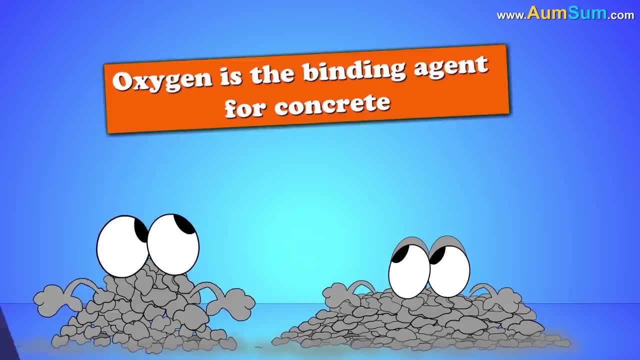 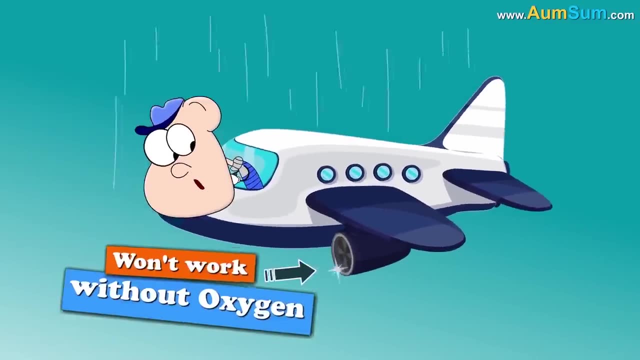 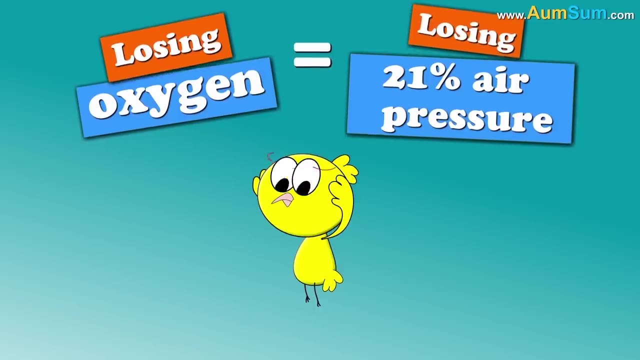 As oxygen is the binding agent for concrete. Cars would stop And planes would fall from sky, as their combustion engines wouldn't work without oxygen. Also, losing oxygen means losing almost 21% air pressure. This would cause our inner ear to explode.